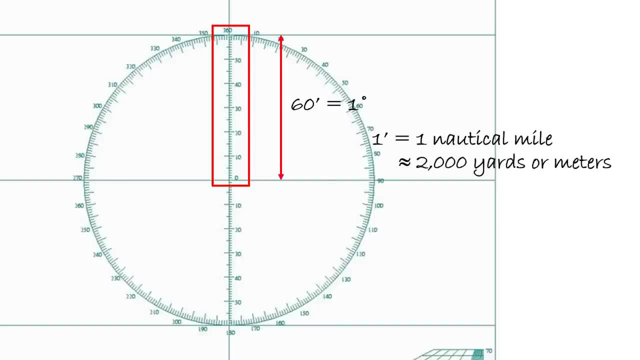 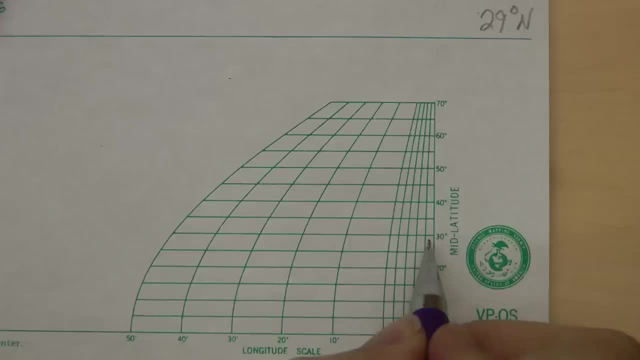 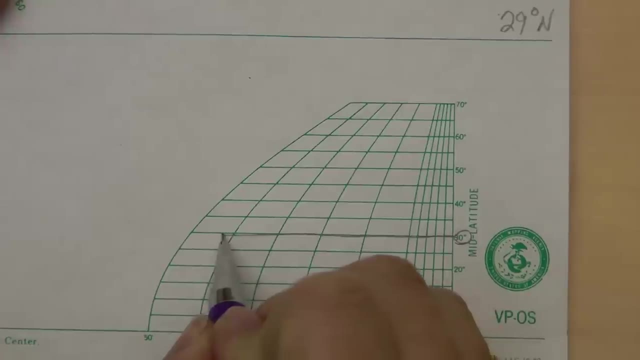 2000 yards or meters. We go to the longitude scale and draw a line on the nearest latitude. In our example that's 30 degrees north. The scale is in arcminutes and since 60 arcminutes equals 1 degree, the entire width of this. 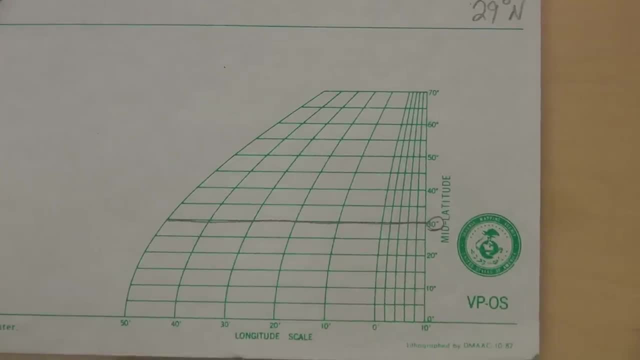 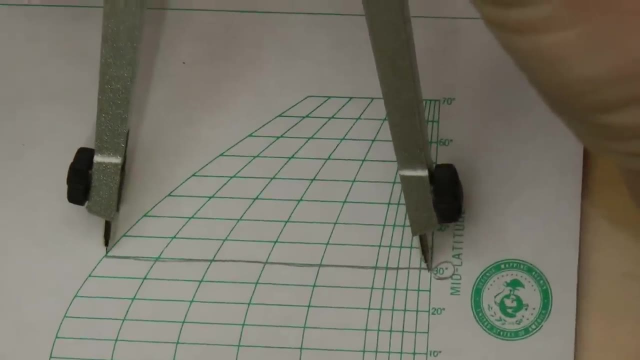 scale at our latitude is the average spacing of longitude in 1 degree increments. Take your divider and set it to measure the width of 1 degree longitude. With your divider set to this distance, measure to the left and right of the center line. 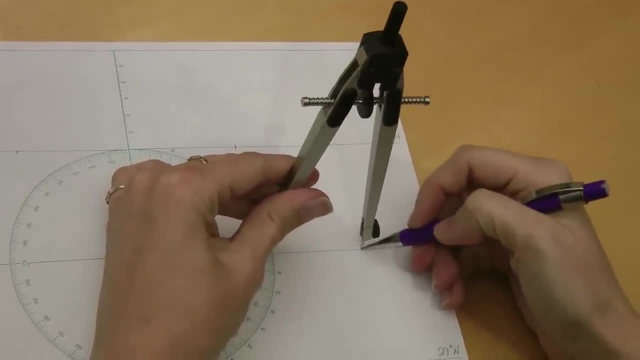 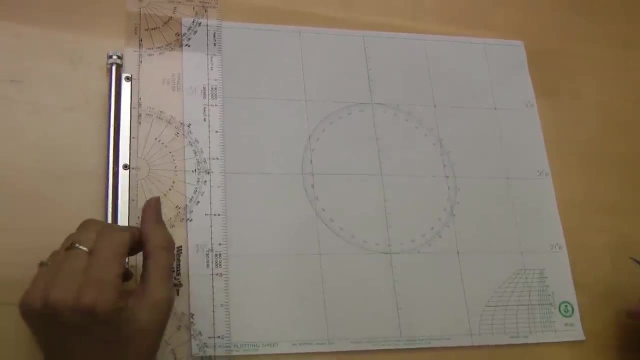 placing two or more pencil marks at each degree increment. Then draw and label your longitude lines. In our example, let's say our nearest longitude is 60 degrees west. As west increases towards the west or left on the sheet we label the left one as 61. 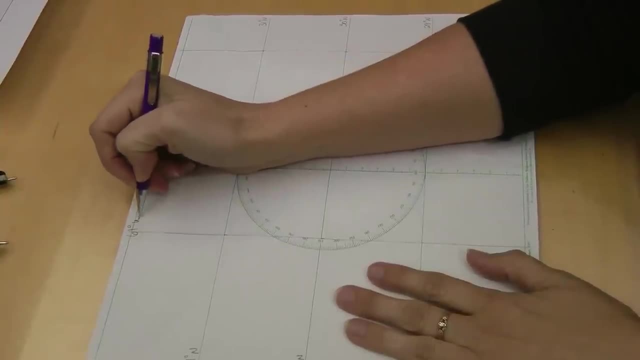 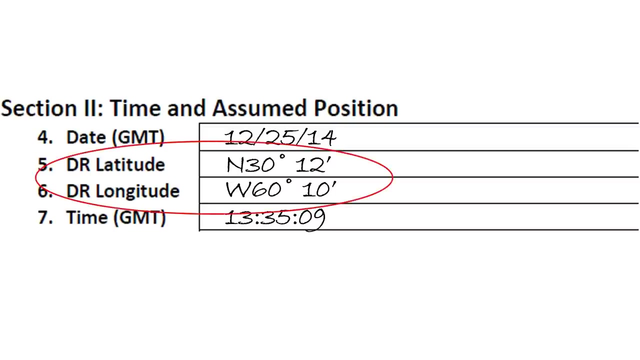 degrees west and the right one as 59 degrees west. Let's say our dead reckoning is 30 degrees north and 12 arcminutes and 60 degrees west and 10 arcminutes. For latitude, remember the angle increases as we go north, so our latitude coordinate. 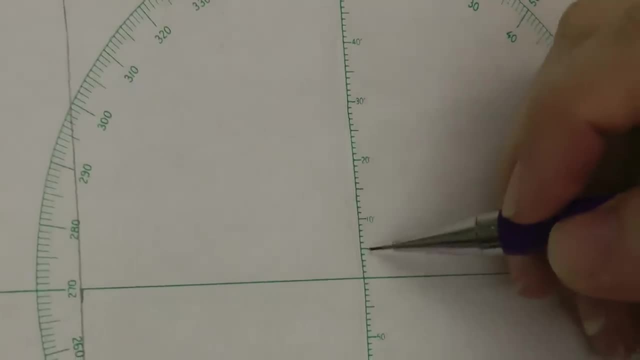 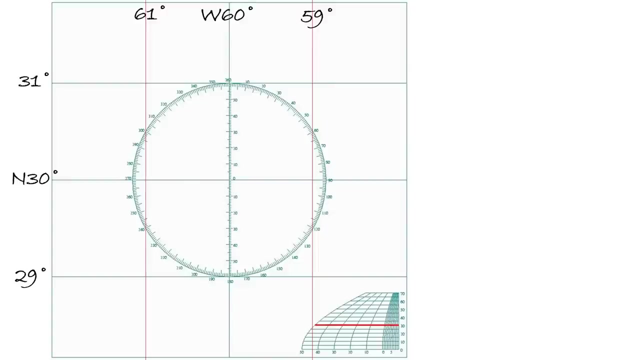 is north of degree 3.. Using the scale, along the center line of the page we put a mark at 12 arcminutes above 30 degrees north. For longitude, we need to use our longitude scale. It's separated in 10 arcminute increments for the first 5 sets, then in 1 or 2 increments. 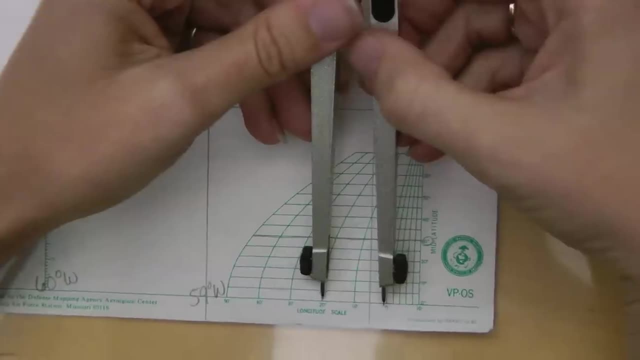 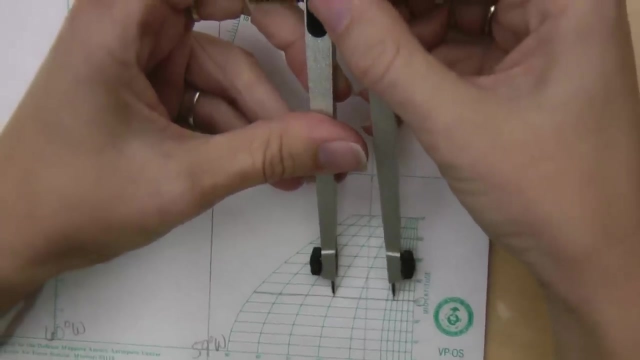 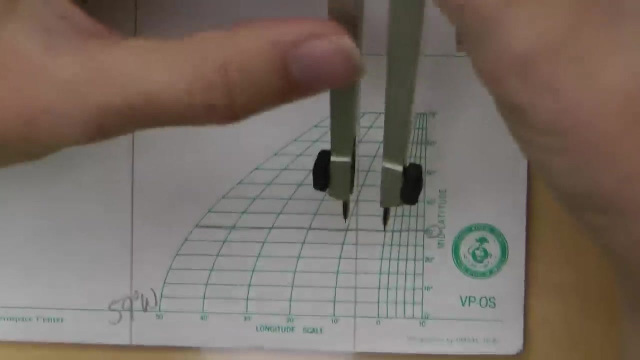 for the last 10 arcminutes. If you needed, for example, 25 arcminutes, you'd set your divider from 20 to 0, then halfway into the 2 arcminute blocks to measure out 25.. In our example we need 10 arcminutes, so we simply measure 10 with our divider. 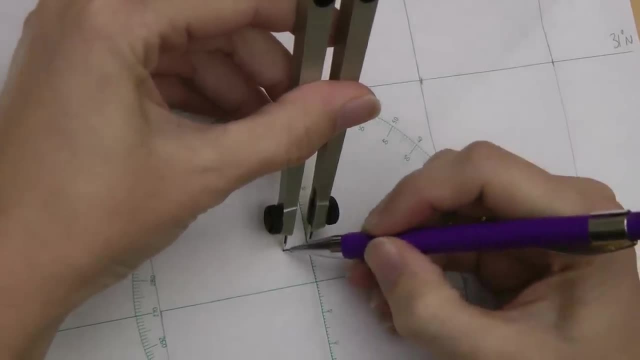 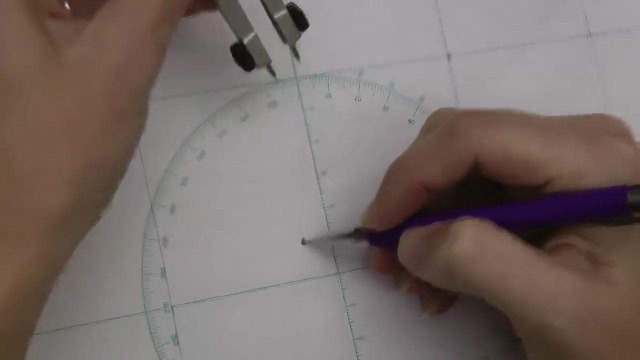 You then move your divider to the dead reckoning mark for latitude and measure out your dead reckoning longitude. In our example our longitude is west, so it increases to the west or left of the sheet. We put a dot in this spot and label it dr for dead reckoning. 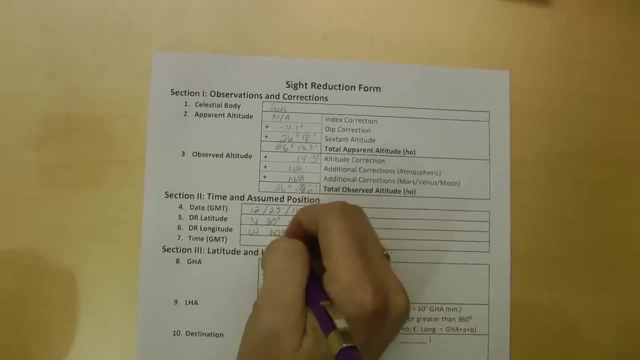 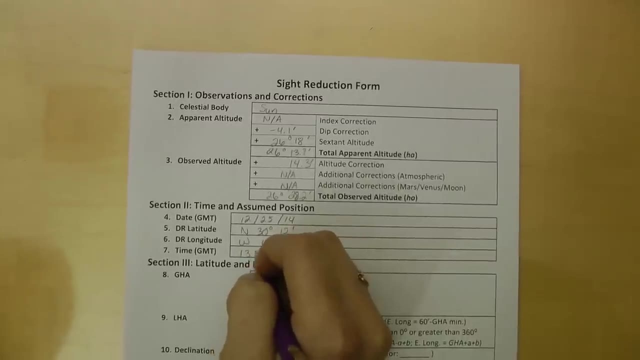 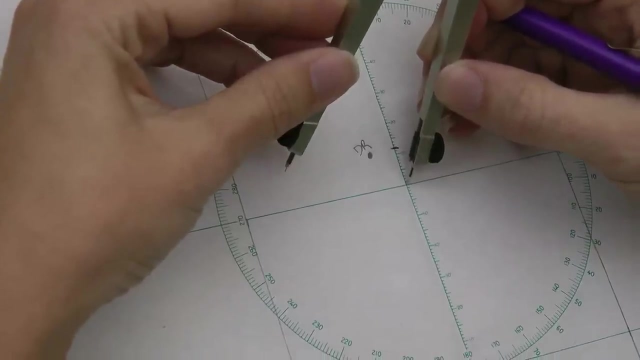 This is our estimated position. In the site reduction form you'll pick an assumed position usable with the site reduction tables. The assumed position is often different from your dead reckoning. Let's say we have an assumed latitude of 30 degrees north, an assumed longitude of 60. 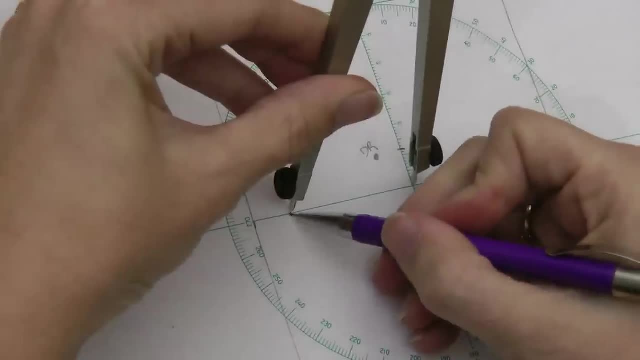 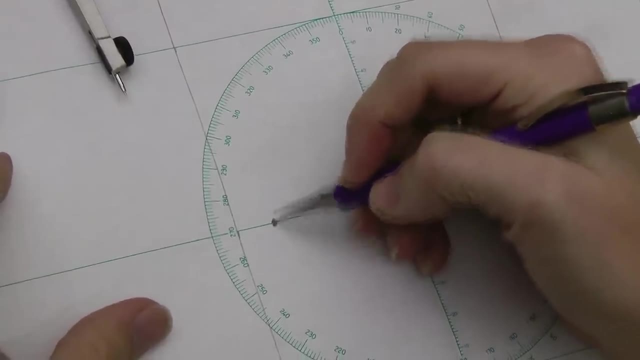 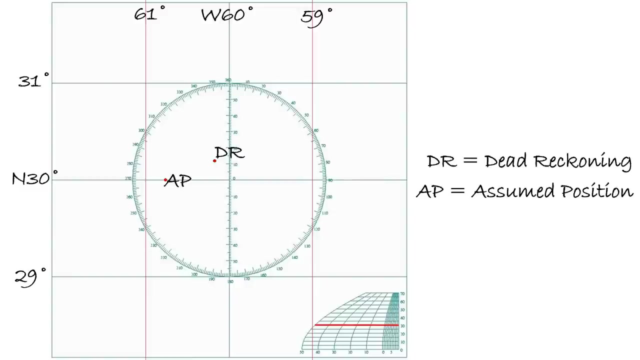 degrees west and 46.5 arcminutes. Using the same methods that we used for dead reckoning, we measure out and mark our assumed position on the chart labeling it AP for assumed position. With our site reduction form we'll have a celestial body with an azimuth angle calculated. 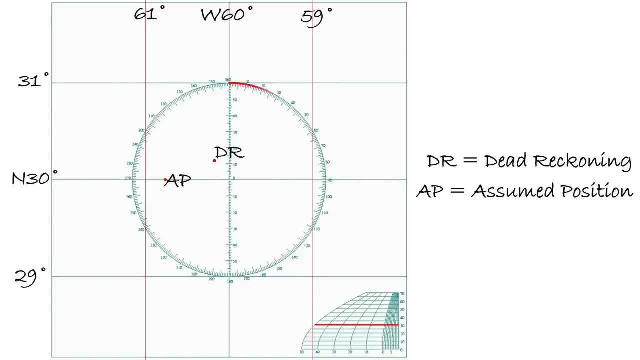 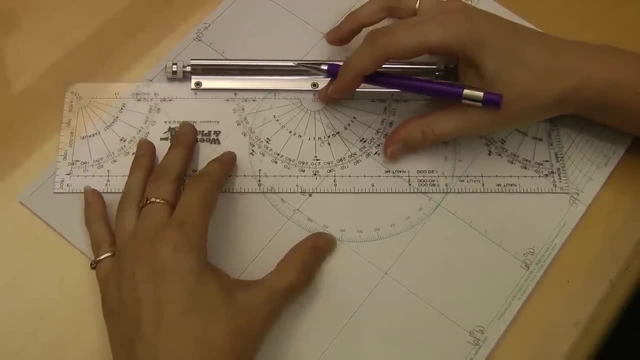 We use the parallel plotter to measure that angle in the center of our sheet using this compass. Then we'll roll the plotter to our assumed position and draw a line pointing to the celestial body. This line will run through our assumed position, pointing towards the geographic position of 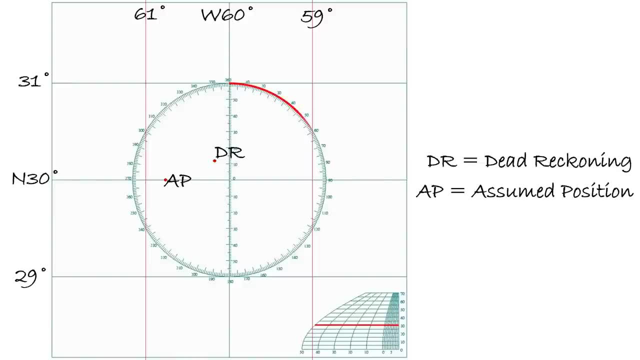 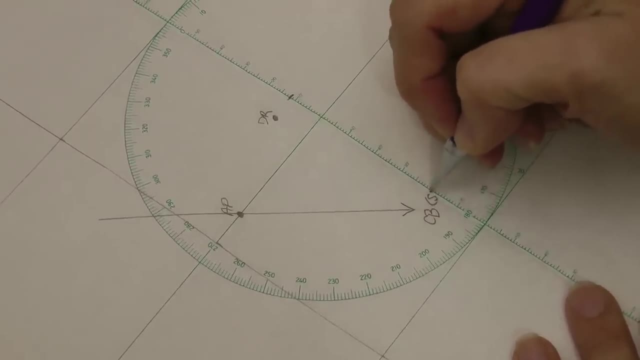 the celestial body. In our example, let's say the azimuth angle is 20 degrees west, The azimuth is 141.9 degrees. This gives us a line pointing to the southeast towards the geographic position of the sun. With our site reduction form, we'll have to calculate an altitude intercept using the. 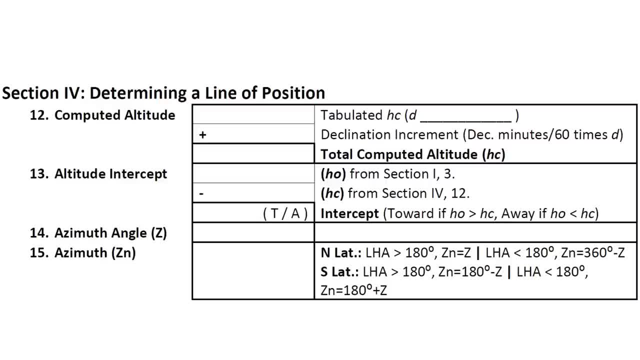 observed altitude, abbreviated HO, and the computed altitude, abbreviated HC. If your HO is larger than your HC, then you mark the distance towards the celestial body from your assumed position. If HO is less than HC, you mark the distance away from your assumed position. 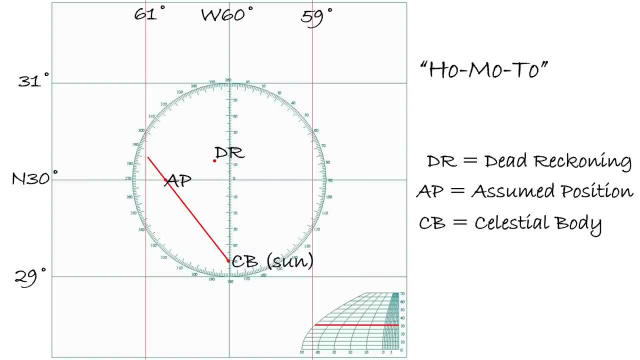 The mnemonic HO-MO-TO helps to remember this rule. In our example, let's say, HO is larger than HC. so the HO-MO-TO mnemonic reminds us that we measure from the assumed position towards the celestial body. Let's say, our altitude intercept is 35.9 arcminutes. 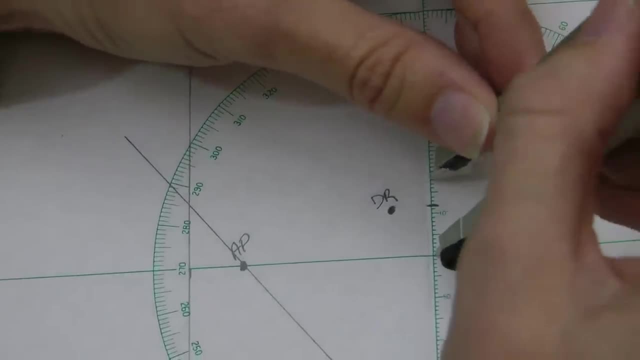 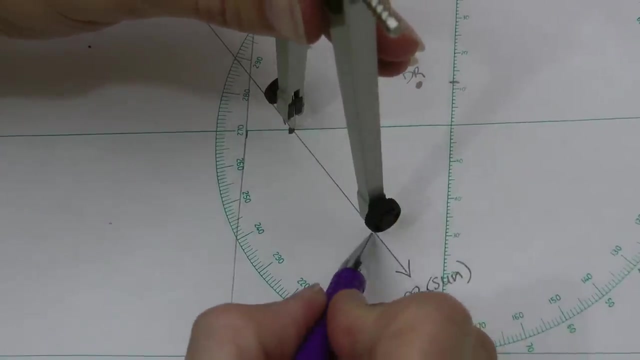 So we use our divider to measure from the assumed position. We use our divider to measure that distance, using the scale on the center line, and mark this position on the azimuth towards our celestial body. The line of position lies perpendicular to the azimuth at the altitude intercept. 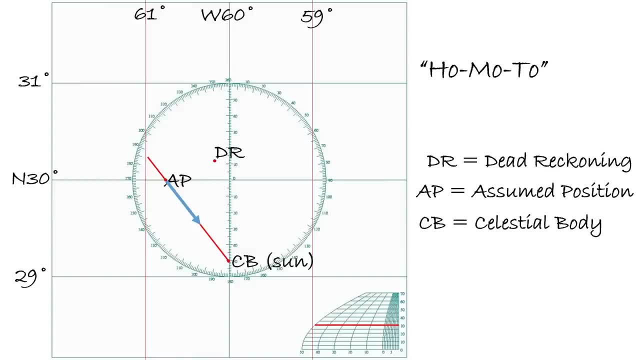 Use a ruler to draw your line of position. In our example we see this places the line here. We label the line of position by writing the time that we took our measurement and the name of the celestial body. Also note LL for lower limb or UL for upper limb when needed. 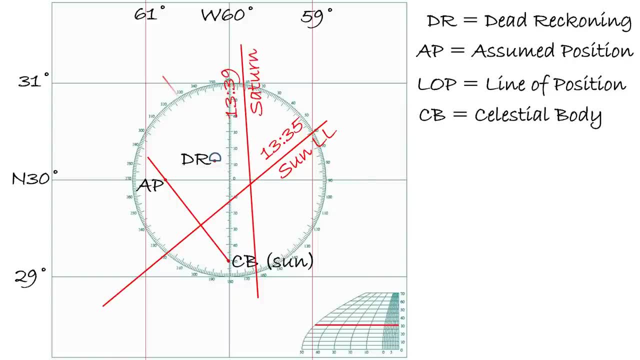 You repeat the process with another celestial body or two, and your actual position lies where these lines of position intersect. You label that position as fix, along with the time and date you obtained the fix in parentheses. In the future, you'll calculate your next dead reckoning by estimating your speed and 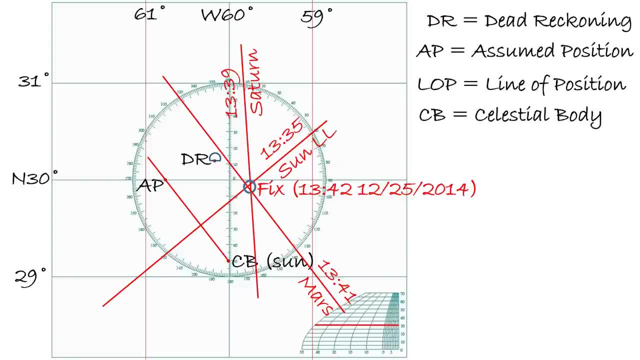 direction from this point and repeat the process. Thank you. In this manner, you chart your position as you navigate. Note that dead reckoning is often marked by a closed half circle. Also, there are some symbols commonly used to mark your calculated positions. 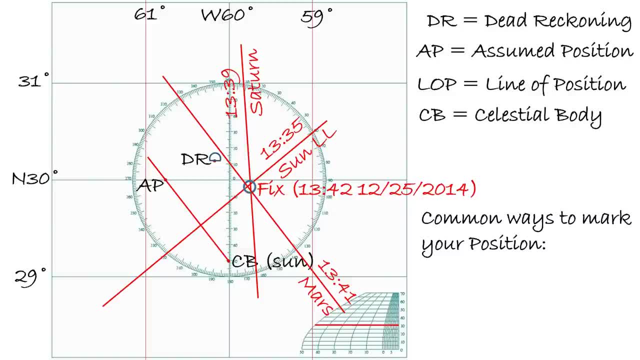 The US Navy, for example, uses the following guidelines: If no more than two lines of position were used, then this is called an estimated position, or EP, and is marked with a square. A circle is used for three or more lines of position and is called a fix. 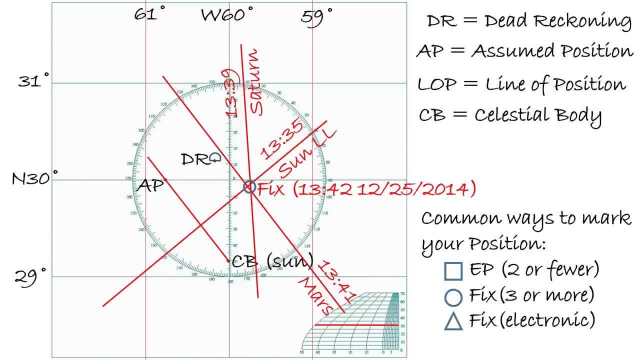 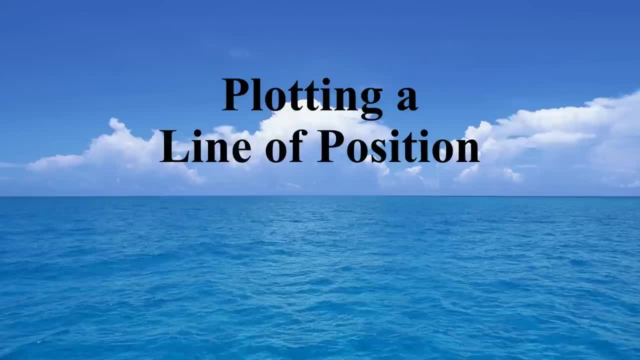 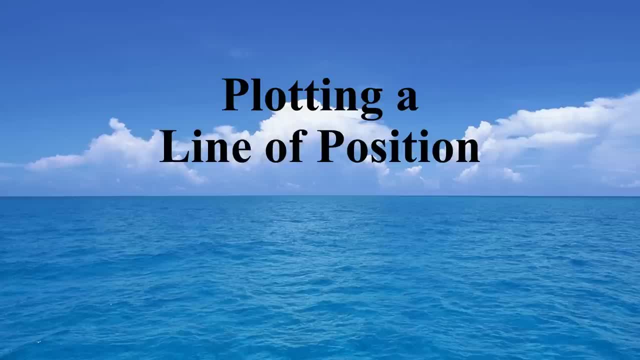 Thank you, Thank you. Oh, are you a pirate or a man of war? He cried. 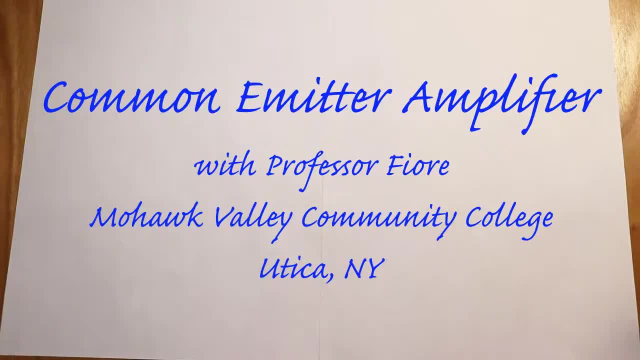 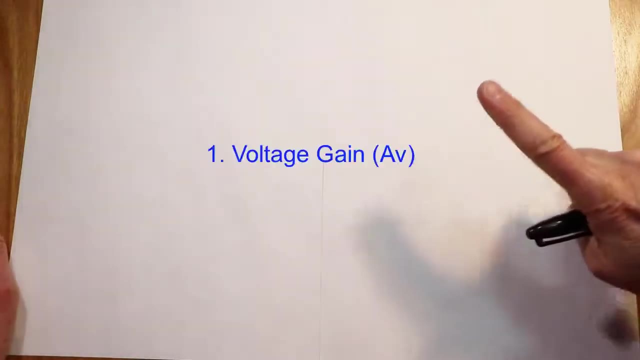 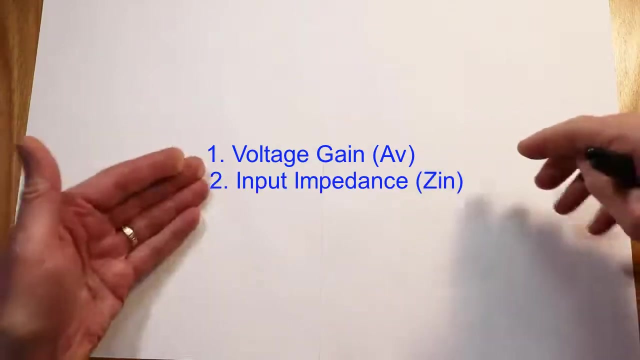 Hello, Today we are going to look at common emitter amplifiers. Yay, We're gonna look at three things on the common emitter amplifier basic configuration. First one, voltage gain amplification factor. Second one, the input impedance. in other words, what does this amplifier present as a load to some driving source, like a microphone, for example? And thirdly,